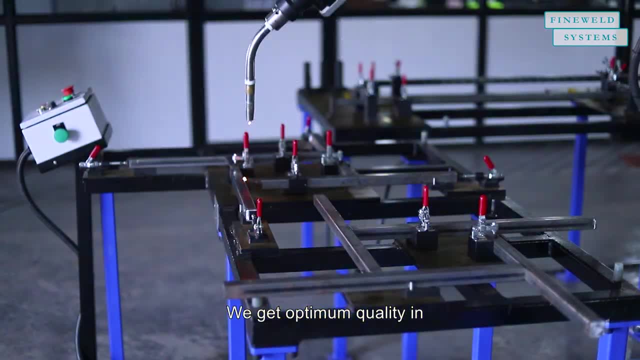 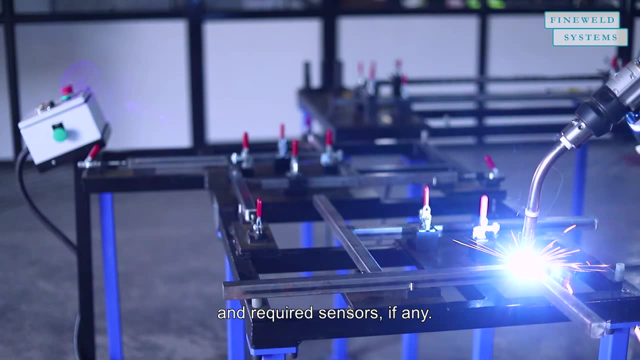 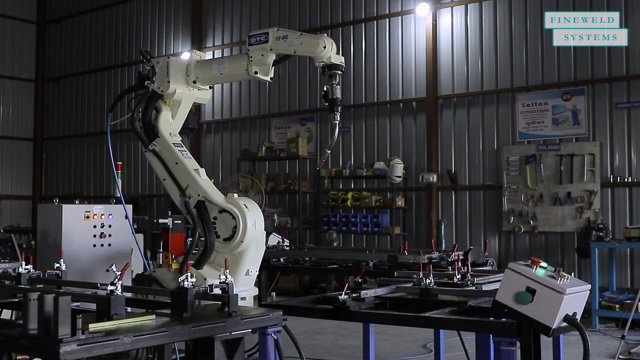 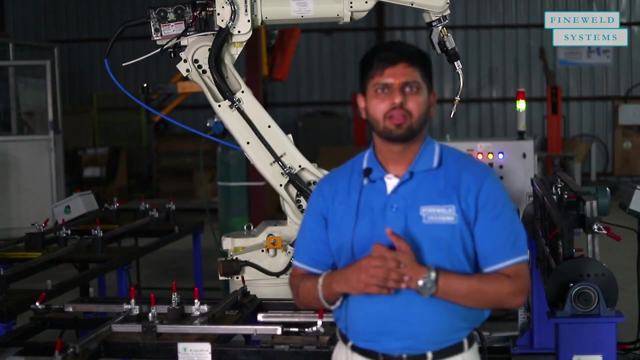 are still the pioneer in that welding also. We get optimum quality in both the thicknesses, be it low thickness or be it high thickness, with our welding power sources and required sensors, if any. So now you can see we are doing welding of 21 and the diameters. You can also see the difference when we look at this part that 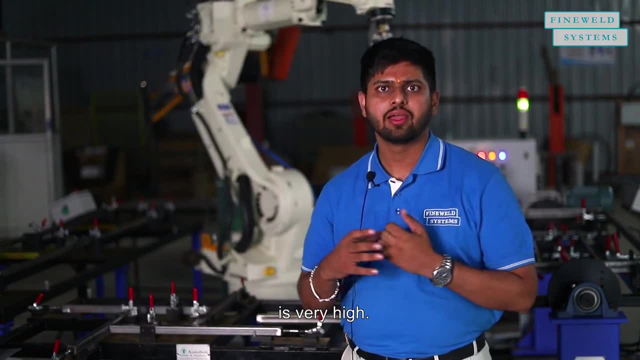 it is obvious on this hand or at this outside side of the motor, the difference is very big. So we are going to do a perfect примерно, just like how the other impl esempos have been puncture flattened. We are just going. 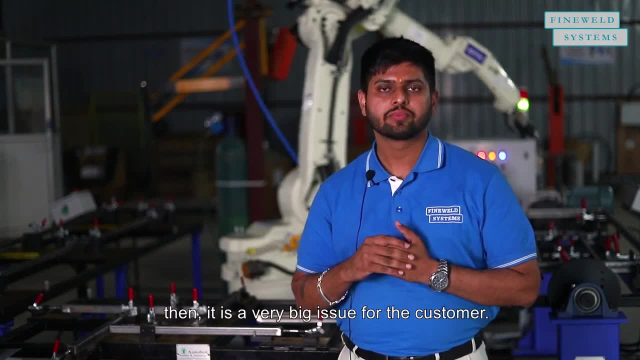 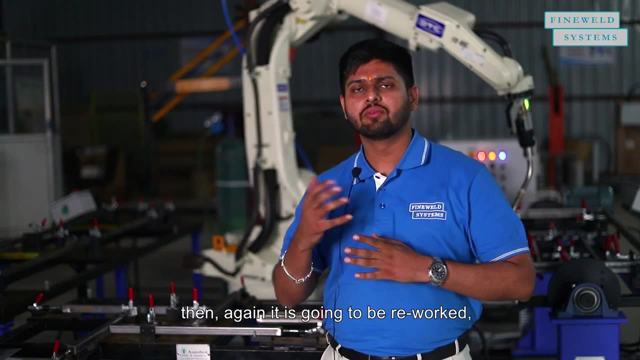 to go through the same part to this end and they seem very much the same. but probably suppose that when um steel welding process we choose, then we have to filled the mortises or fully filled the deste as well. Then we also create some holes where all parts are. 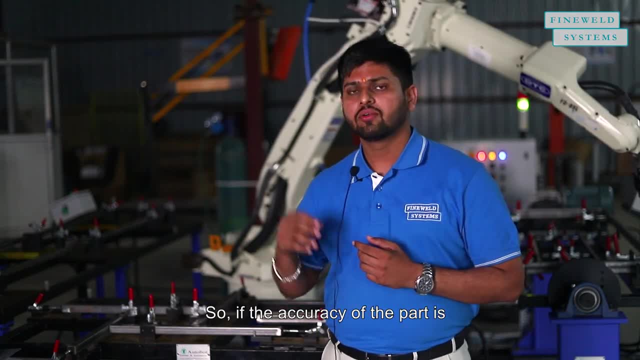 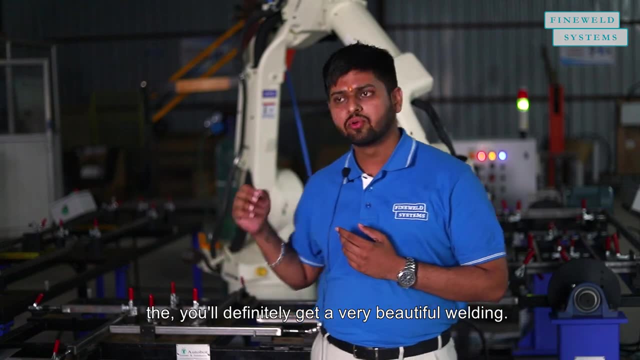 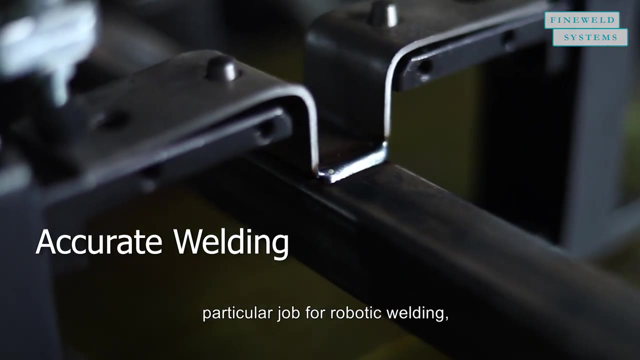 making such a beautiful welding robotic cell. so if the accuracy of the part is correct and it is in the limit what is required, then you will definitely get a very beautiful welding. as you can see over here now, there is a basic thumb rule while selecting a particular job. 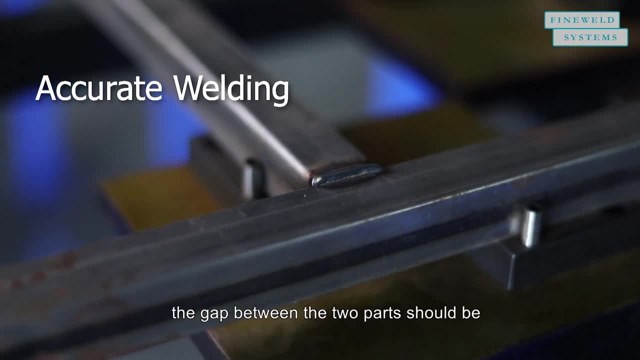 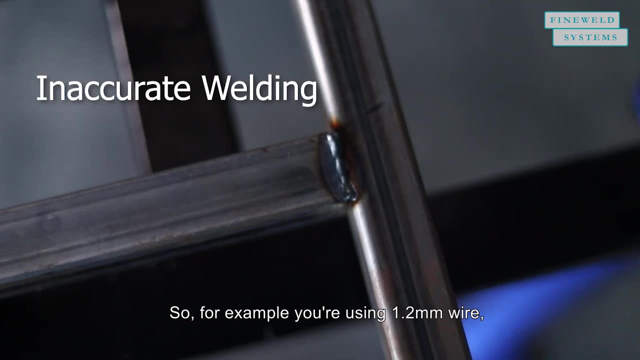 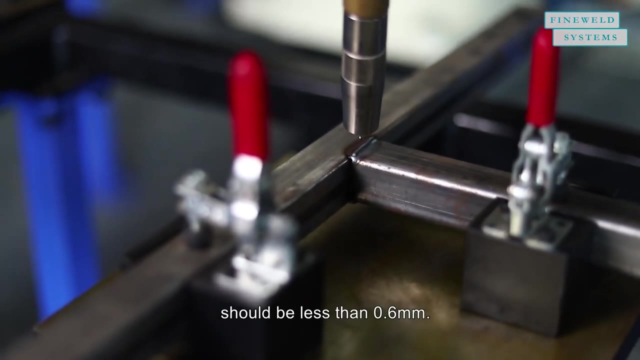 for robotic welding, when you are joining two parts, the gap between the two parts should be half of the diameter of the wire which you are using for welding. so, for example, you are using a 1.2 mm wire, then the gap between the two parts to be welded should be less. 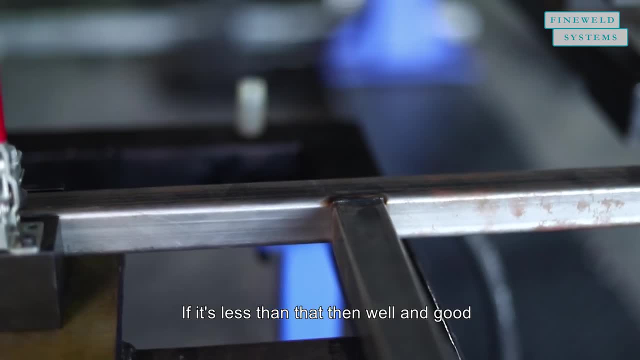 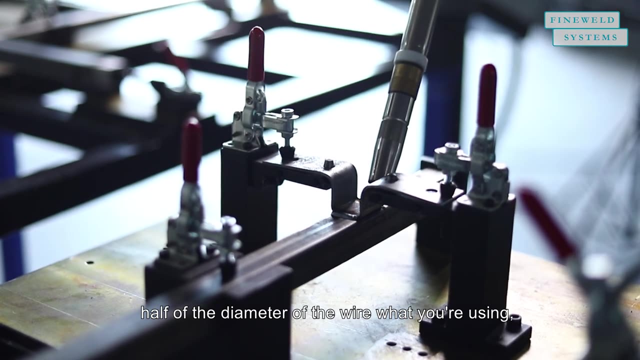 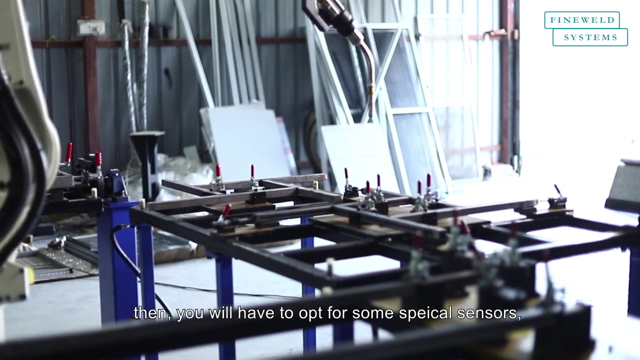 than 0.6 mm. if it's less than that, well and good, but it has to be less than that. if it is more than the half of the diameter of the wire- what you are using, then welding is very difficult to do. in that case, then you will have to opt for some special sensors. then 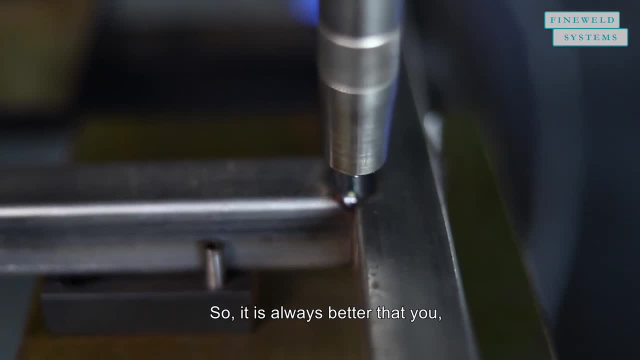 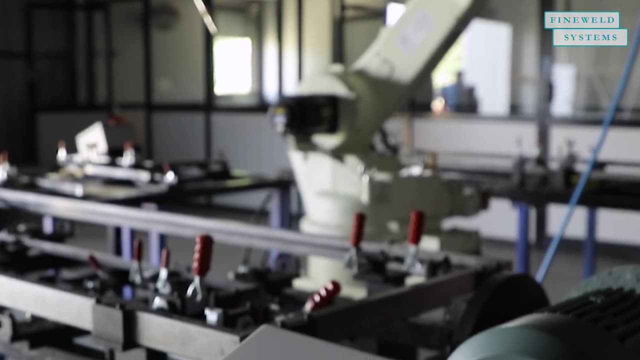 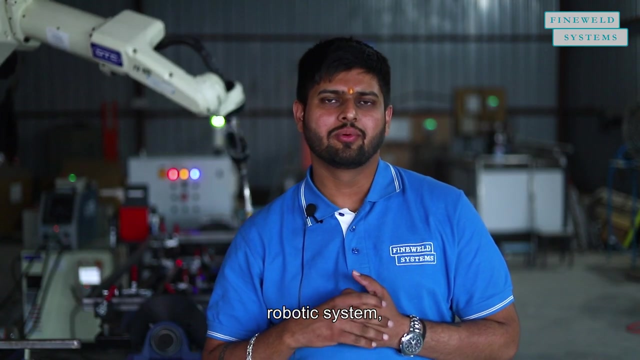 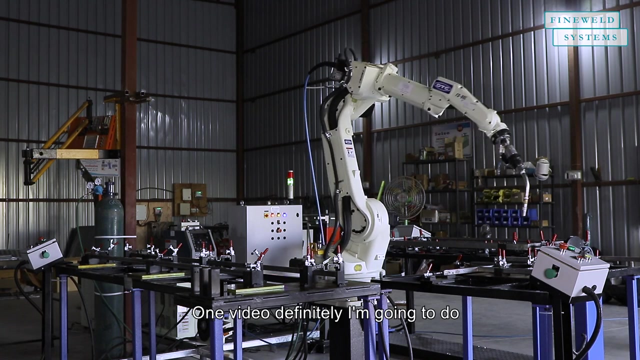 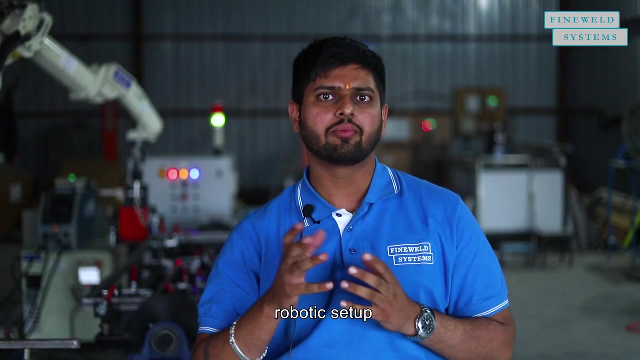 it is a costly affair, so it is always better that you correct your job and then you opt for a robotic welding. now, in this particular system- robotic system- we have used three fixtures along with manual clampings. one video, definitely, i am going to do for this particular thing, that how to select a robotic setup, or how to select a.